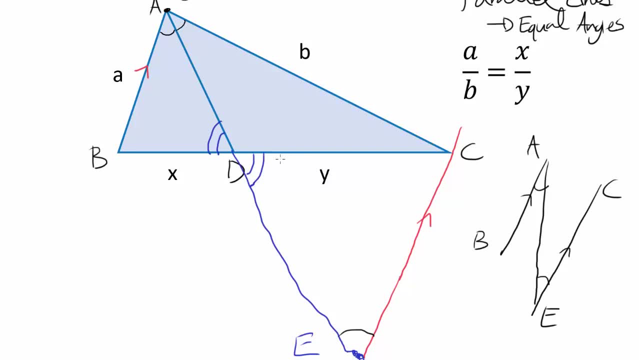 a, d, b being vertical angles with angle c, d, e. So these two are the same And, and obviously we have a parallel triangle that's popping up, you have triangle a, d, b and triangle and triangle c, c, e, d, because you have this angle being equal to this angle and this angle being equal to this angle, you have a, a, So, by a, you have triangle a, d, b and triangle c, c, e, d. 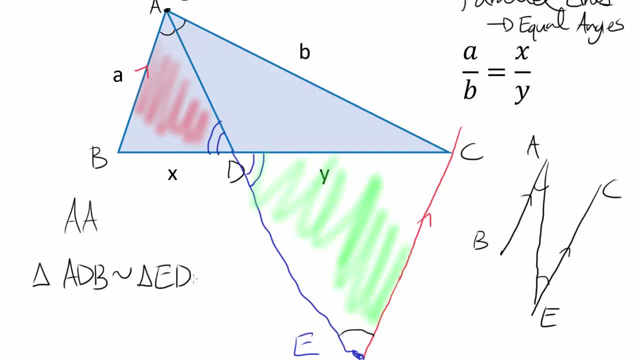 Being similar to triangle e, d, c And because of that we can relate the ratio of corresponding size of these triangle. So we have a divided by the corresponding corresponding part. in this, this green triangle is e, c. So right here, e c, let's just let this be k. So we have a over k, being equal to x over the corresponding part, y. So, using the ratio derived, 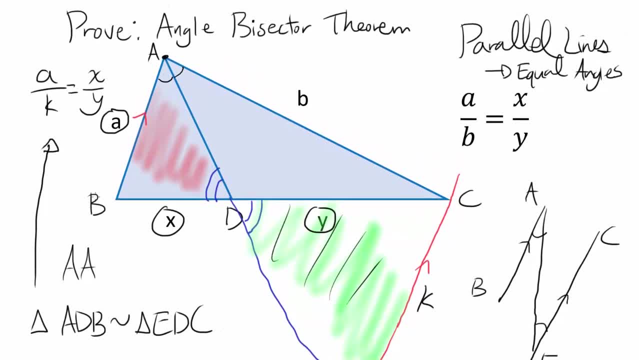 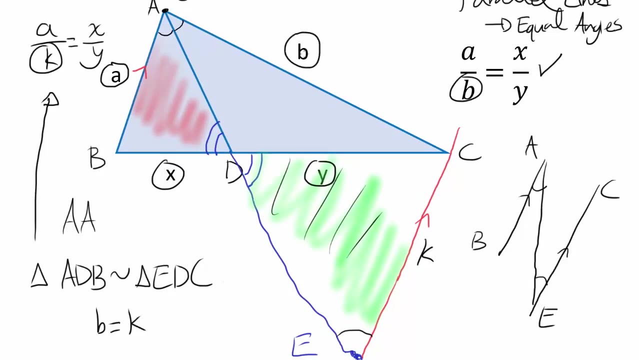 from the similar triangles. we have a over k being x over y And we are very close. we want to prove a over b is x over y. So if we can show that b and k are the same, So if b is equal to k- remember b is this side and k is this side- we are done Because when you replace this k with b, you have what you want: a: b over a, b, a over b is equal to x over y, which is angle c. 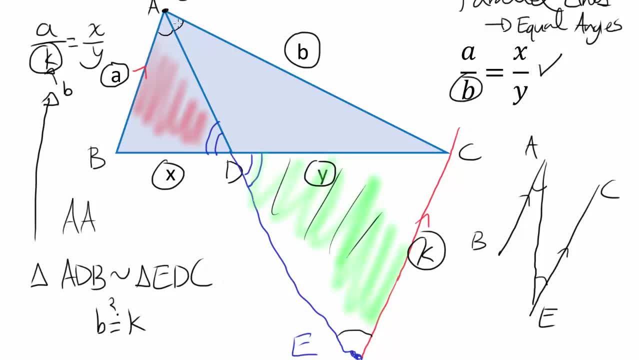 And how can we do that? Well, focus on this. you have this angle, angle c a d, being equal to this angle, angle c e d. So, triangle c a e, this yellow triangle, this yellow triangle, this entire triangle is isosceles. this entire triangle is isosceles because this angle is equal to this angle. two angles are the same in this triangle And that's telling you this triangle is isosceles. 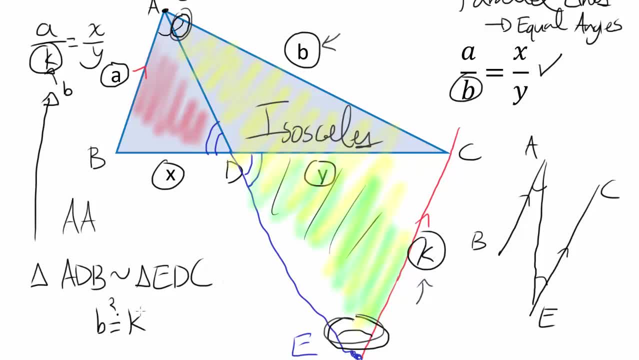 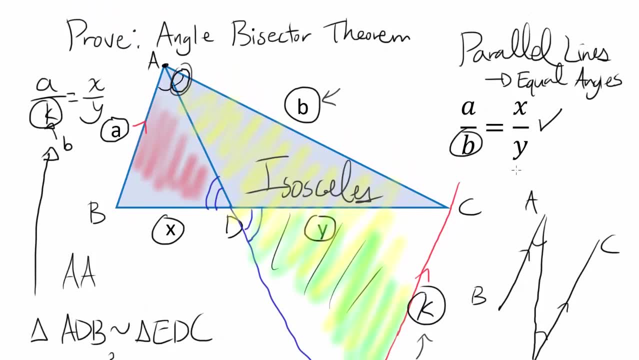 side b and side k have to be the same, or b is equal to k. and that's telling you a over b is equal to x over y. and stating it another way, we have proven the angle bisector theorem.